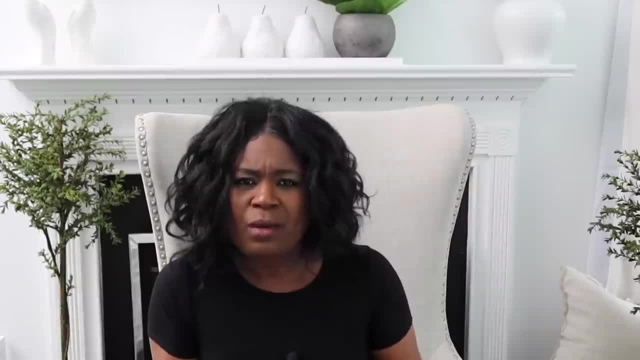 such a huge part of our life that it's important that we live it in a beautiful way, And in the book I share with you some really just out of the box tips and tricks and kind of guides and things to really help you implement that, whether you work at home, work in an office or truck. 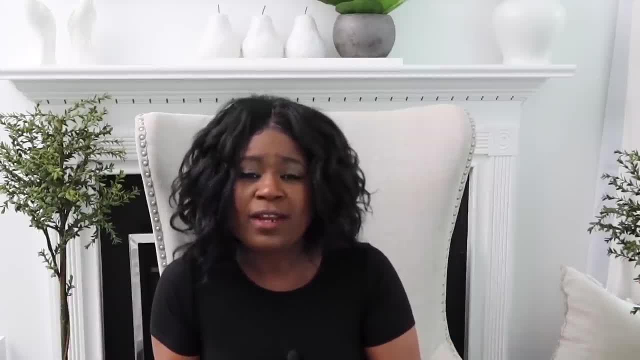 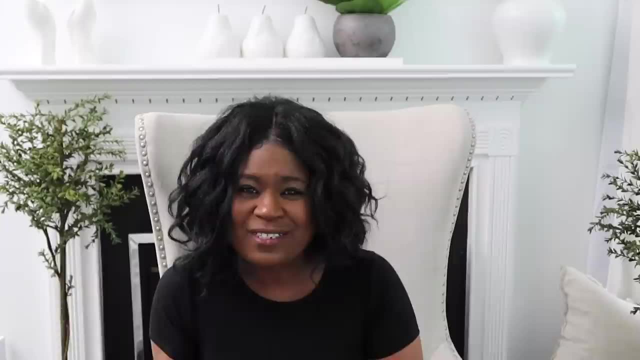 driver work in a hospital. it really is for everyone and their work life. So, again, it's available for pre-order. I'll put it in the description box below. So now let's get into those tips. So, friends, I do understand that it can be difficult to get your child on board with. 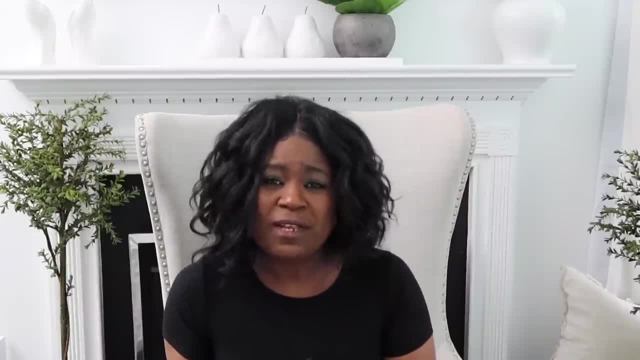 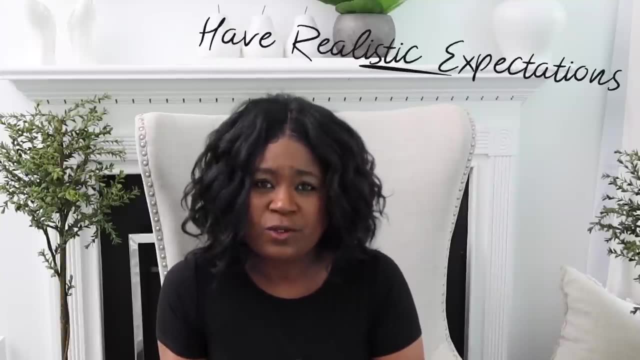 keeping their room orderly. It can be frustrating, but the first tip that I want to share with you is to really have realistic expectations, because one your child's space, that to them is their sacred space, That's their safe space, And we want to be careful not to invade that space, or 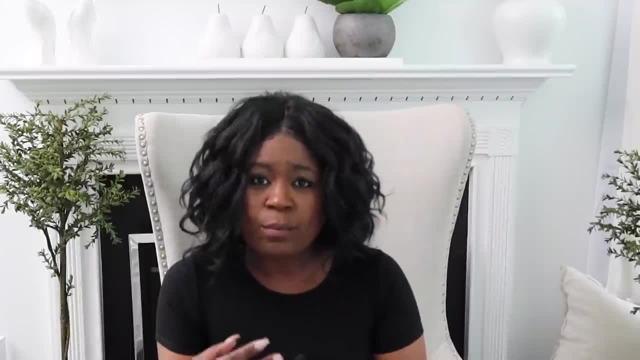 just kind of be overbearing with it, Or we want to have our approach so that it really gives them power when it comes to their things and their space. So we want to. when you're going into creating any rules and expectations, you really want them to be. 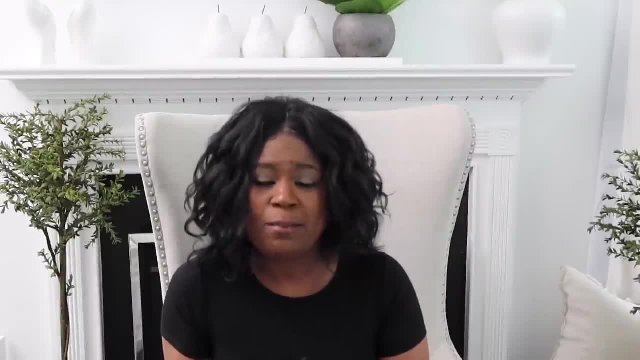 realistic. My second tip is to set a good example. You know kids, oftentimes they don't listen half the time to what you say. They listen to what you do, And so you can easily, you know, start the process of remedying yourself from the frustration of your child not keeping their space in order. 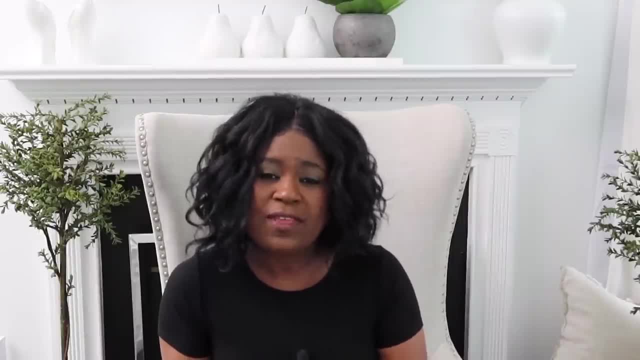 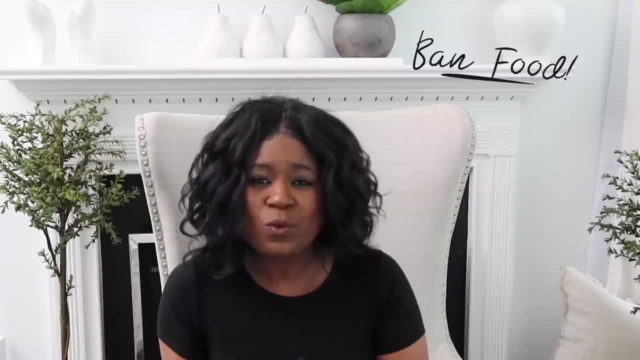 to be that example, picking up your things, keeping your things tidy, you know, be that example for your child. Tip number three, friends, is to ban all food from the bedroom. This is the one of those things where it's a it's a health hazard if you don't implement this. sometimes, if you have, 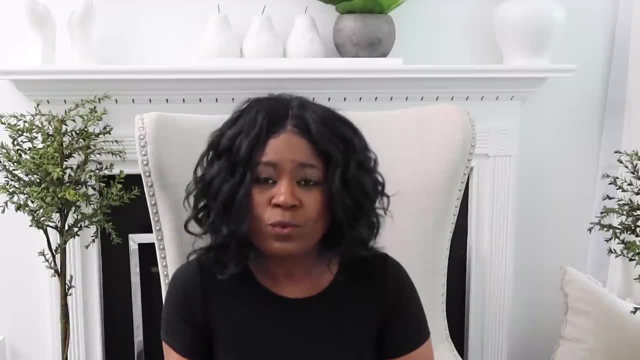 that really messy teen or kid. So one quick kind of a rule that you can establish within the home is, you know, only water in the bedroom, no food or you know or other drinks, And that really can give you a sense of security, even if there is clutter in their space. 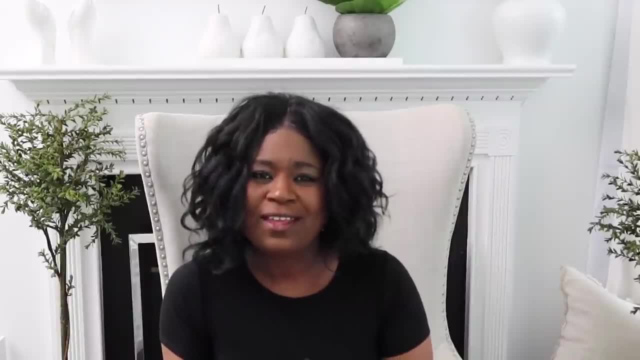 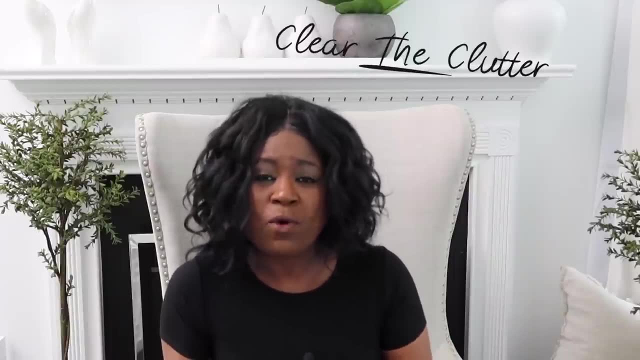 that there's no kind of health hazards going on in the room. So tip number four, friends, is to clear away the clutter, And so the less that there is to deal with, the easier it is to keep maintained, And so one thing that you can do is, as a family, incorporate a routine where 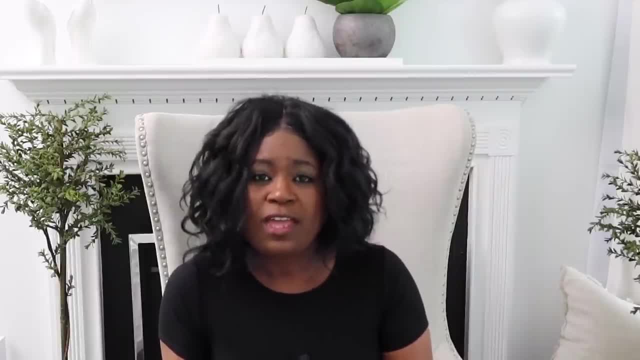 you have a family routine of purging, So it may be kind of one day a month that you all kind of commit to pulling 10 things or 20 things from your space that you need to donate, And then everyone runs and gets their things. And it's kind of a way for again leading by example. 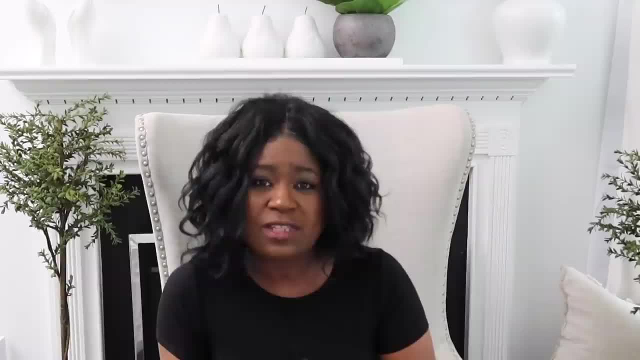 but having the opportunity to get your kid to really purge some of those things out of the room, with giving them control of what they will purge out of this space, So that can be a great way to do it when you implement it as a family. Now, another thing that I do want to say is: you want 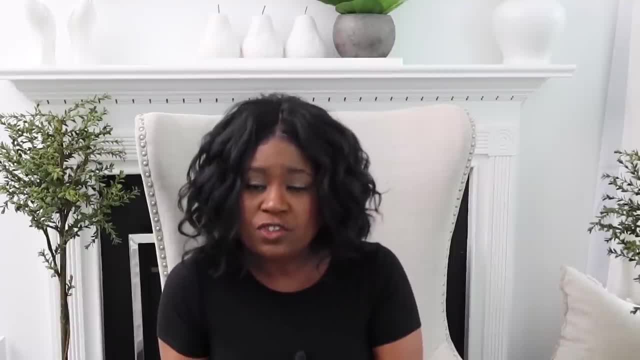 to give the control of where their things go to, to the, to the kid, to the teenager, to the child. So if they're giving up their items, you know, ask them like: how would you like, who would you like to get this, Where would you like to take this And tell them the options that are out? 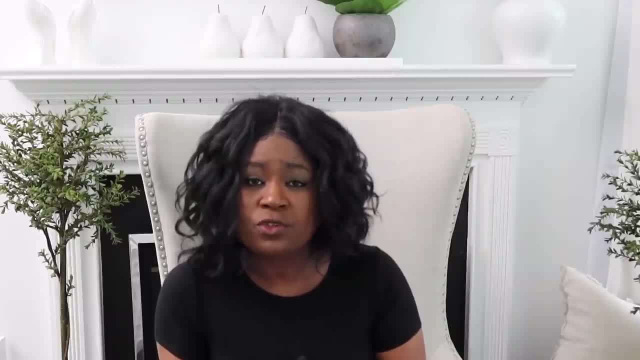 there. This is a great teaching opportunity for your child, a great way to kind of start the process of um, kind of raising them up to be givers and and kind of giving them the information they need that they can take in their life, of how they can purge their items and where they can take. 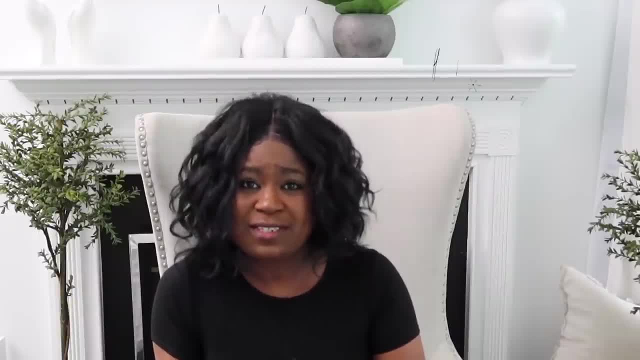 their items. Tip number five is to have systems. You got to have those organizational systems in place in their room. So, even if they switch it around or or they change it, you want to work with your child to make sure that they have a place for. 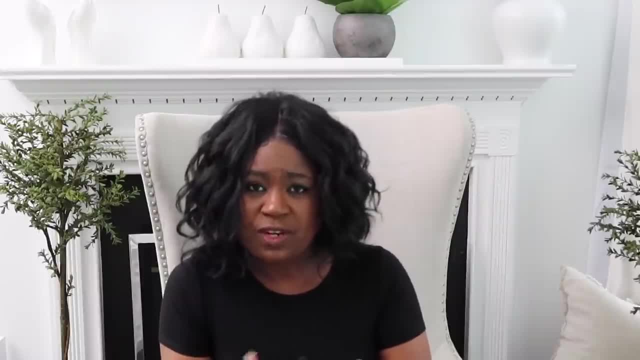 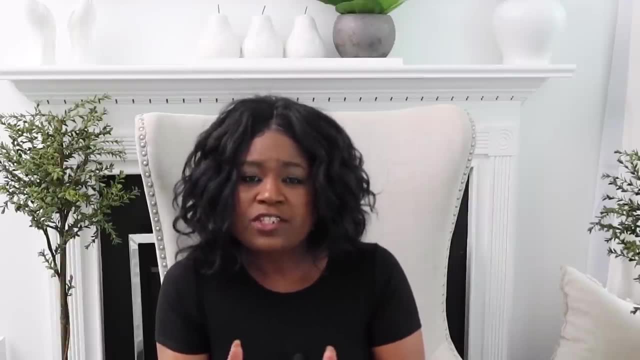 everything in their room. So, for example, sometimes I work with kids within a family because the parent feels like if they bring in a professional organizer to work directly with the child, they will respond better, And so the first thing that I do when I'm working with that child- 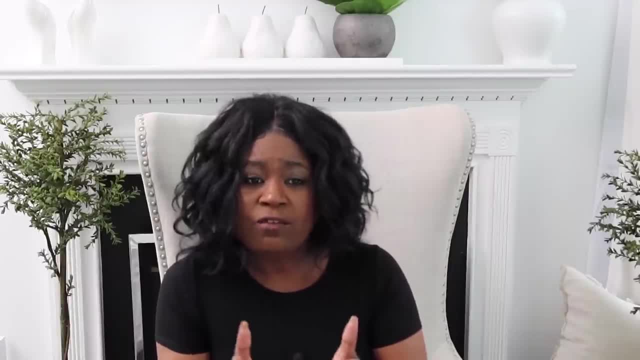 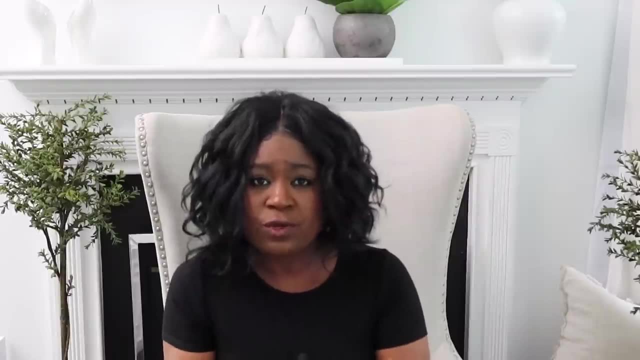 is we walk around their room and we identify kind of where all of their things are going to go, So, for example, their bedside table. you know they may have three drawers. and they'll say, okay, you have three drawers here, And when we initially open it it is probably kind of everything papers coming out of here. 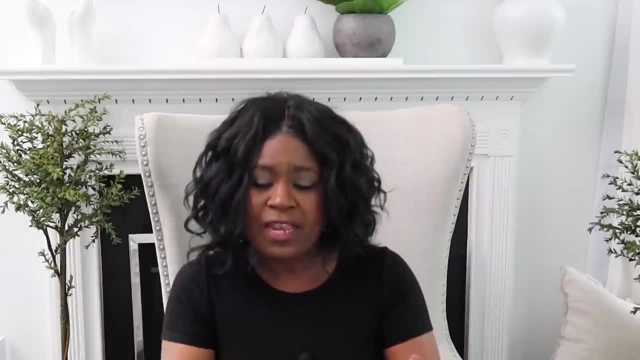 books and little cars and toys, But then what we do is we take everything out and then we name each drawer. Okay, This is going to be the car drawer. This is going to be the book drawer. This is going to be the candy drawer, which you're not going to have candy in the room. 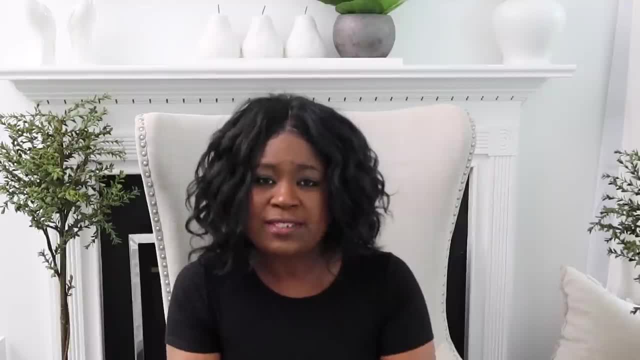 but let's just- I'm just using that as an example, but each drawer has a name, And by taking the time to really not do it for the, but walk them through, taking everything out, resetting it, naming it- They're a part of the. 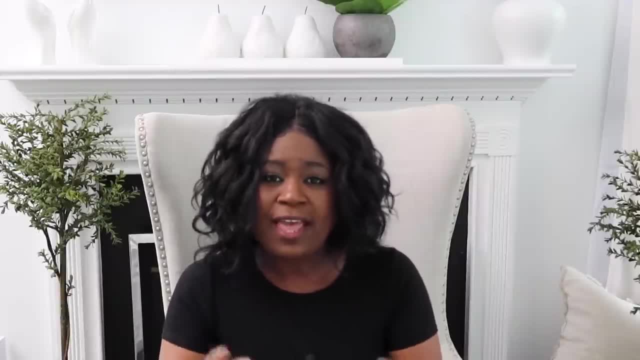 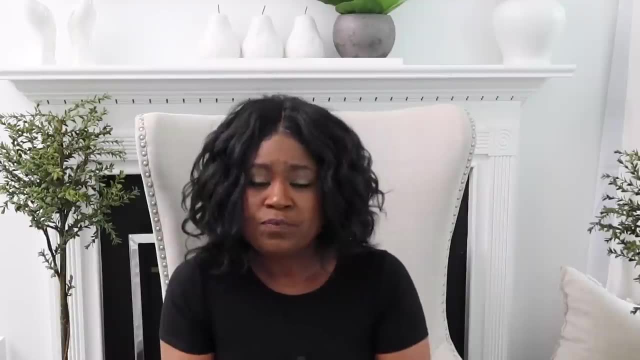 process, which they are getting bought into it And they clearly understand: okay, this is my drawer for cars, This is my drawer for this. So I think that if you really, even if you don't bring in a professional, even if you don't bring in a professional organizer, and you do it yourself, 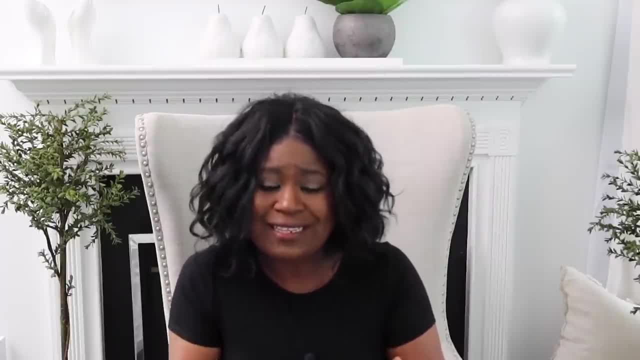 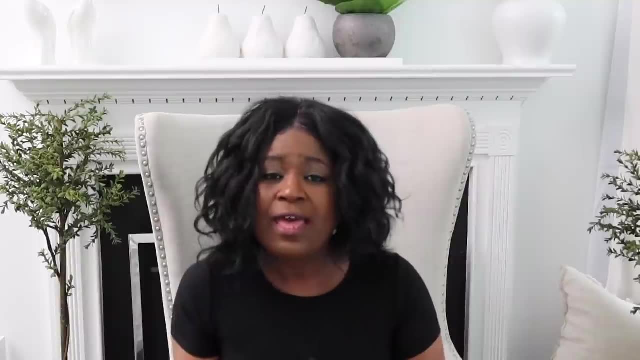 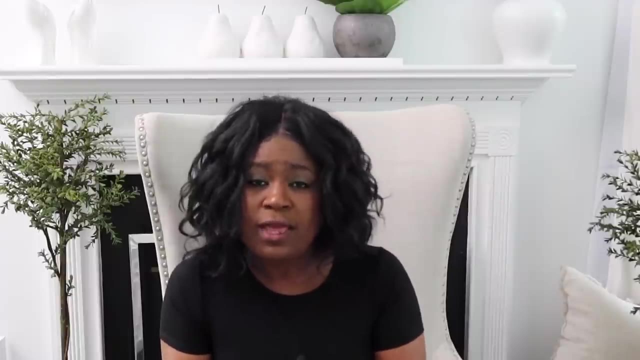 then that's a great way to set that system in place. So go through your child's room with them and make sure they have those initial systems. Then you can back off and let them maintain the systems. And I do want to put out there: my services are virtual, So no matter where you live in the world, if you want me to, 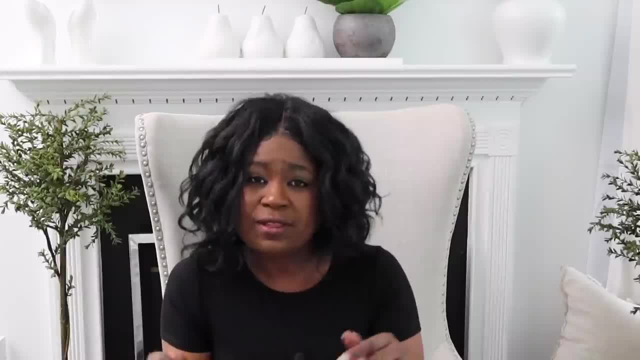 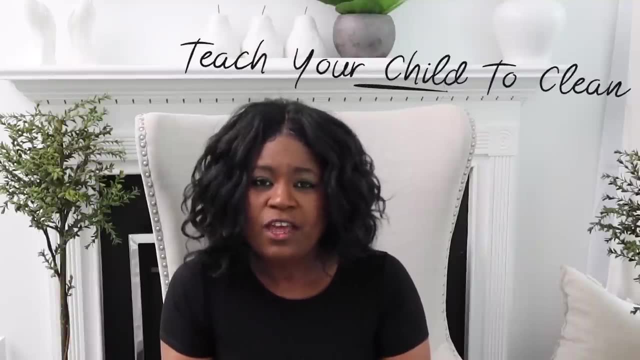 come and assist you and your family with your organizational needs. I'll put the link in the description box below so that you can definitely take advantage of that. Tip number six, friends, is to teach your children how to clean. You know, oftentimes we'll give kids expectations. 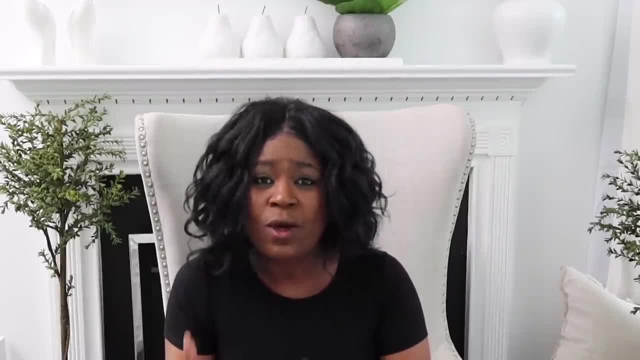 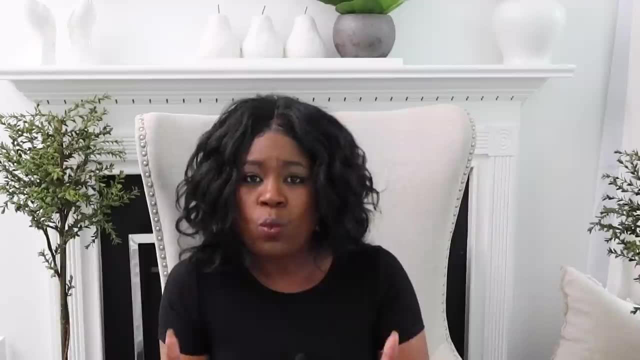 but we really haven't taken the time to really show them in detail how to execute. So you know you tell your kid go clean your room, but have you ever really gone in and shown them what that is? You know you ever have your husband. 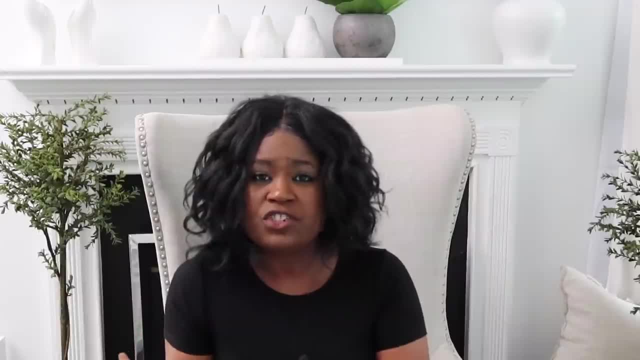 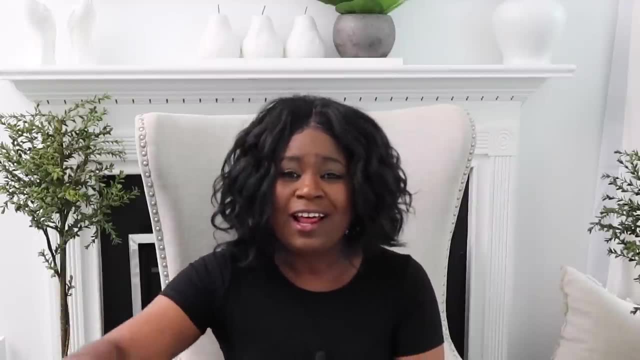 go and wash the dishes and he will do the act of washing the dishes. But you know there are so many other things that go into play when it comes to washing dishes. There's cleaning behind the faucet. There's cleaning wiping down the kind of dishwashing liquid. There's wiping down the. 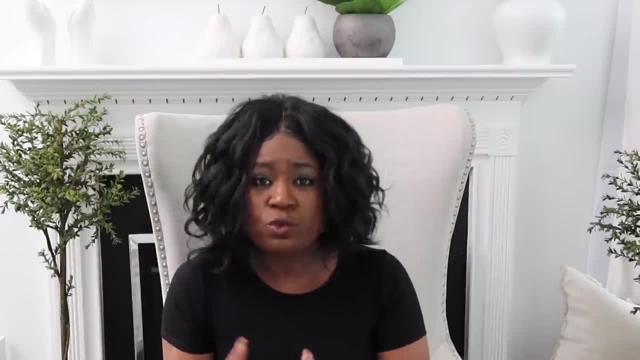 counters, And so if you give a family member expectation of just go do the one act, they may not know how to execute And then it makes you frustrated because you're not doing the one act. You're thinking they're just not caring or they're not doing it right, And that's not the case. So 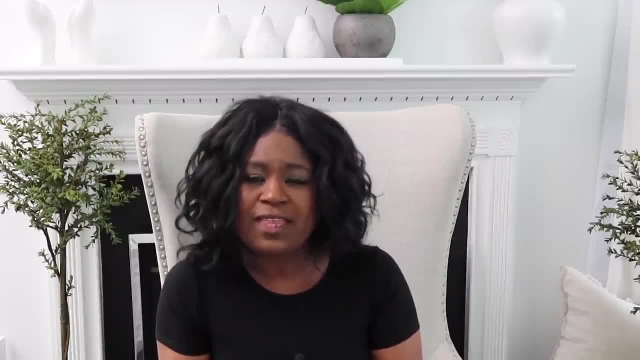 if you, with your kids in their space, you want to make sure that they understand how to clean, and cleaning can be taught so early. You can teach your kids little things early on, like when they're four and five they can start learning how to fold towels. That's such an easy. 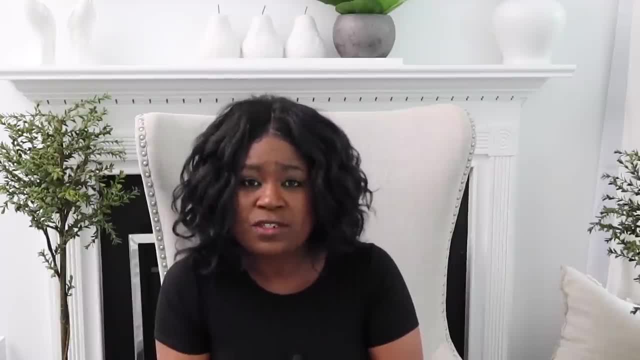 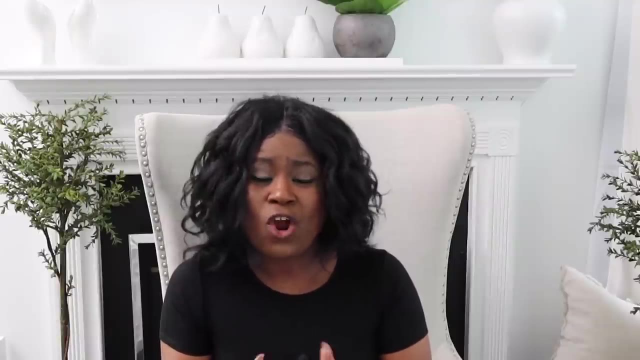 task, And at that age they are like sponges, They want to help, They're taking in everything you give them, And so that is the perfect time to really teach them how to clean, So if you're, and they can really take them all the way into their adulthood. And here is the thing: Kids today 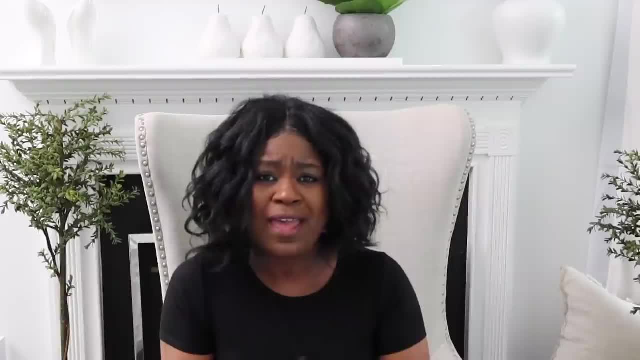 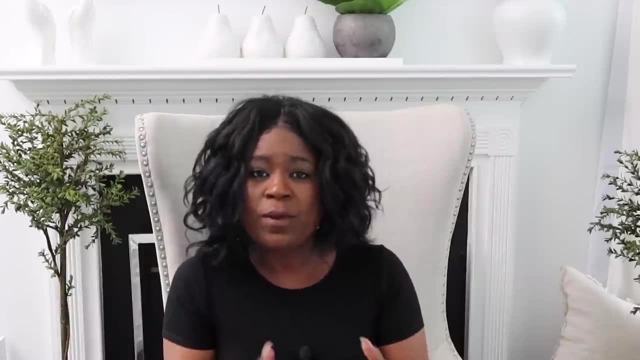 are so smart, They know how to work that technology- the iPads. they can do it better than we can. So that tells you that they can fold a towel and they can keep their space clean and they can help maintain the home. So you definitely want to start early If they know how to turn on. 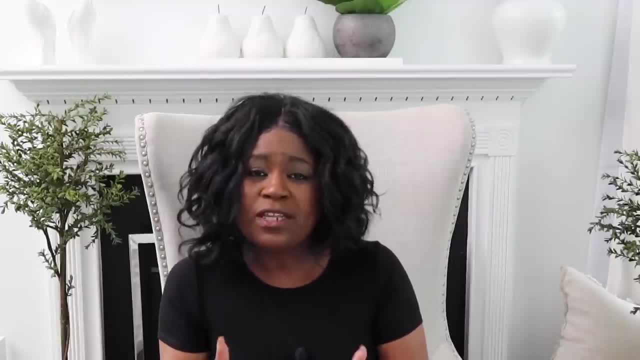 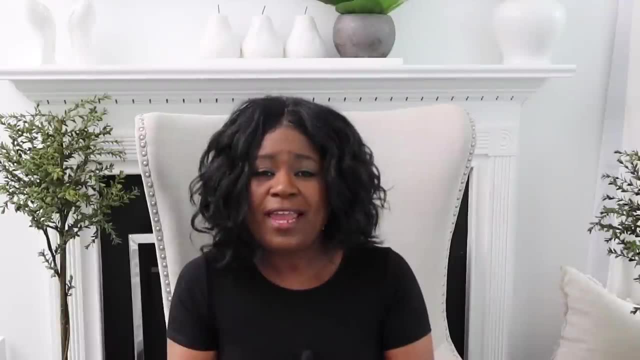 that iPad. they definitely can know how to fold a towel. So you want to definitely start your kids out early learning how to complete that. So if you're a child that's learning how to clean of, take care of the home that they live in. So tip number eight is to do regular maintenance. 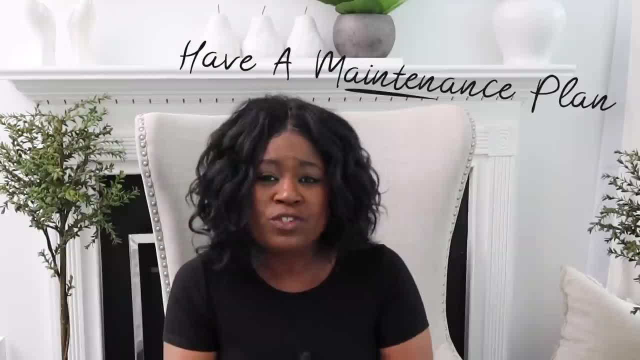 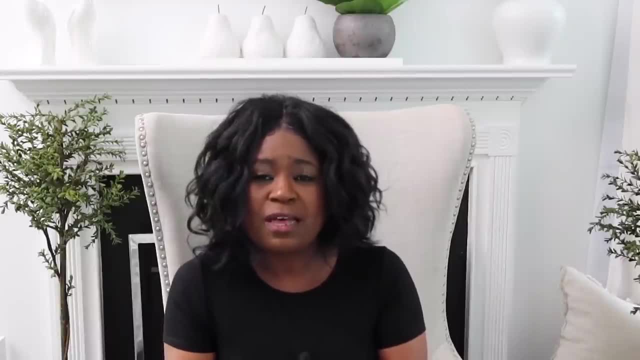 You know you don't want to just kind of leave your kid at it in the room, just never has a kind of maintenance plan. So if it's the family expectation is every Saturday morning everyone gets up and clean their room, then that's the expectation It may be every day when we get up. 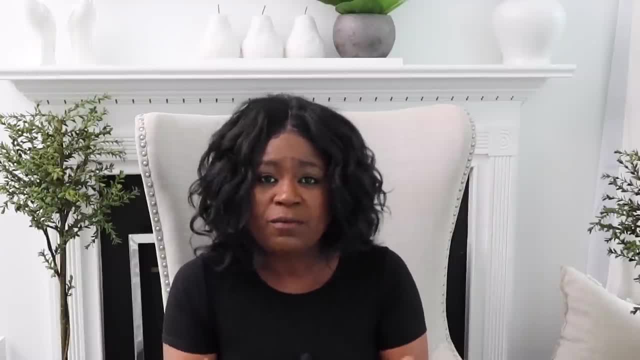 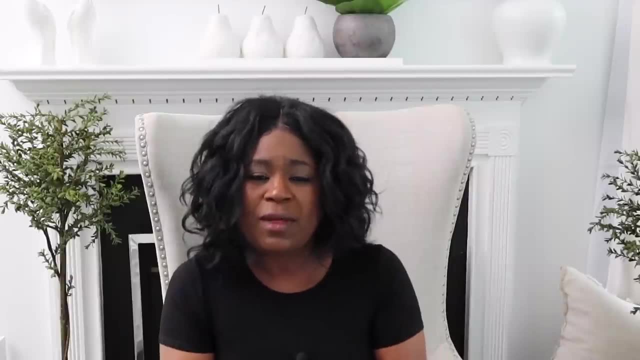 as a family, we make our bed. It also could be at the evening before. at nine o'clock, the family stops and we do a sweep of the home. Everybody picks up their items, everybody cleans their room, and then everybody can go back to their evening or go to bed, whatever the case may be. So 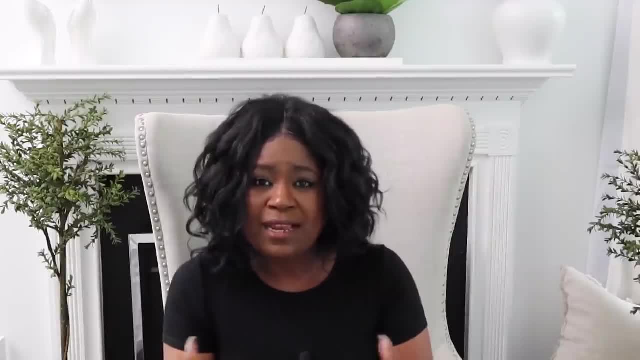 within your home. you want to be sure to set up that maintenance for not only their space but for the entire home. Tip number nine, friends, is to get your child's input. That is so important because that's how you help them connect to their space. You know when you're choosing those. 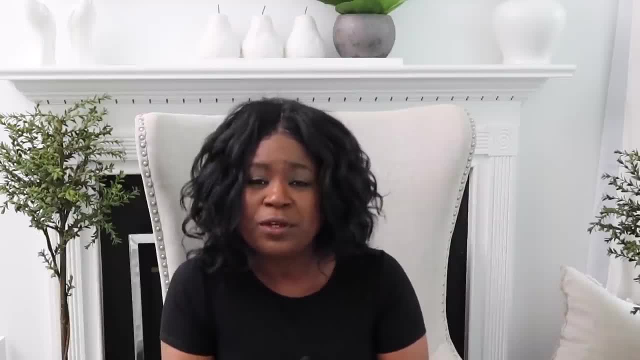 organizing systems. when you're decorating their room, you know, get their input because then that gives them the power to make the decisions And it also gives them the buy-in to keep it in order, because they've decided what bin that they're going to use to organize their 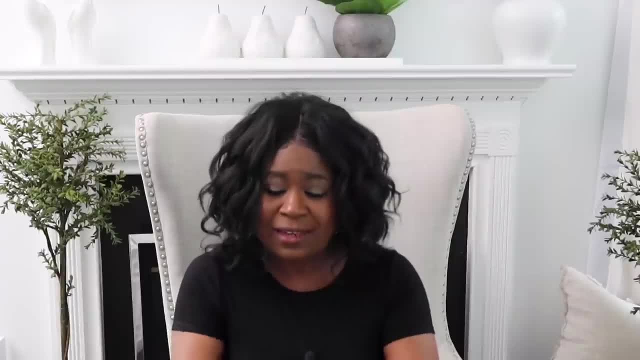 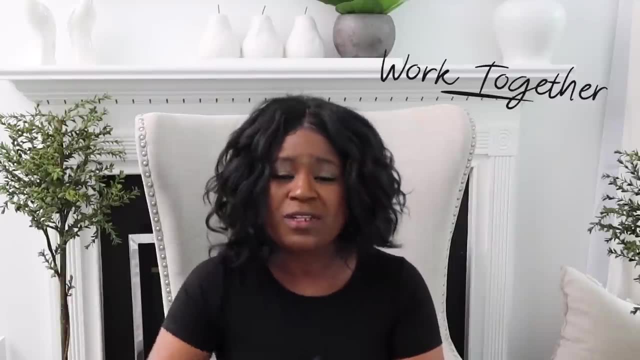 socks, So they know that the socks go there and then they're going to have that buy-in to put the socks there. Tip number 10, friends is to work together. You know, sometimes you'll walk past your kid's room and you're like get the room clean, and you keep going. 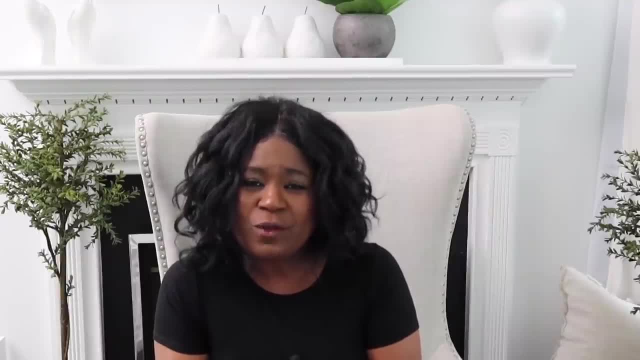 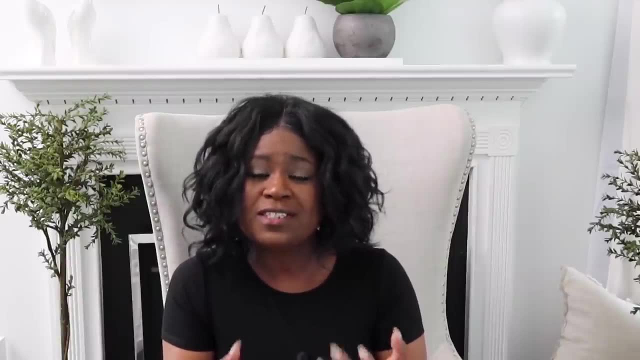 Well, what I want to encourage you to do is to take, you know, some opportunities to actually go into your child's room and clean their room with them. This gives you the opportunity to kind of assist them with learning how to clean their room. It gives you time with 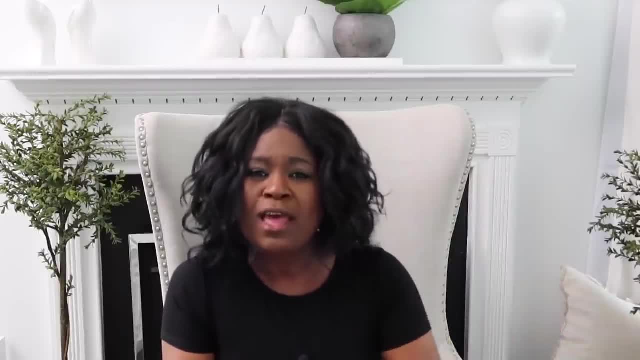 your child outside of them, sitting on across the room on the iPad, but you're really kind of working together. It's bringing that unity. You can even also do it as a family, So you can have a schedule where you alternate days where all of the family goes to one family member's room. 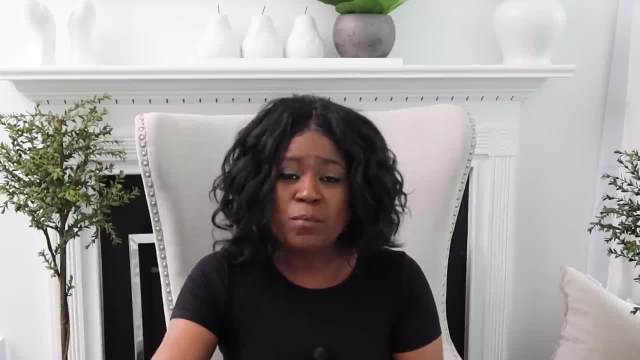 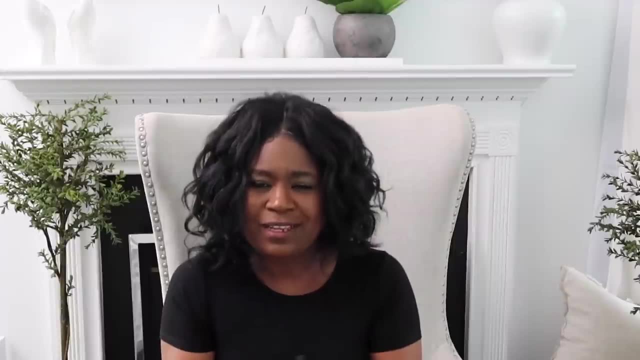 and as a team, you clean the room. So that may work in some families and it may not, but that is something to think about, if you can implement that in your family. I always like to think about cleaning in numbers, So I feel like 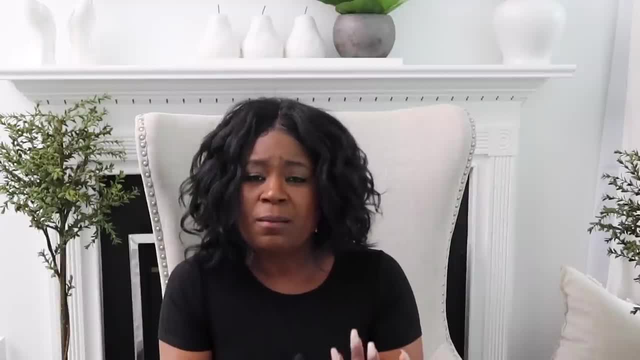 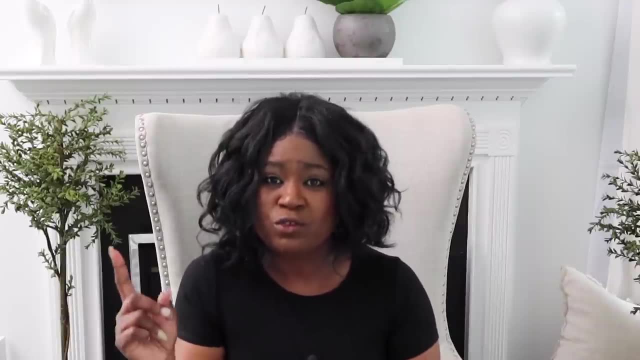 if you have one person cleaning a room and say they're going to do it for 15 minutes, if you have two people cleaning that room for 15 minutes, that's actually 30 minutes because you have two people. 15,, 15, that's 30 minutes worth of work. You add on a third right You 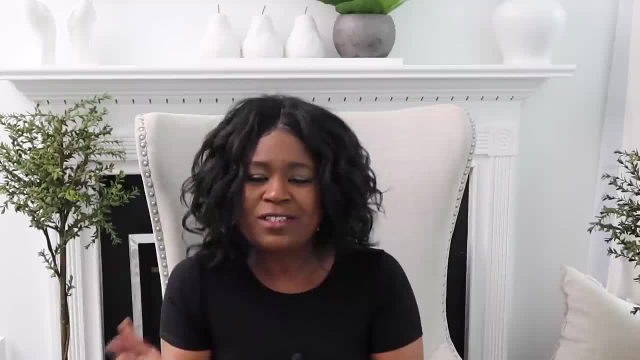 got 45 minutes. So for every member that's, you're adding on double the time. So that's a great way to get a lot done in a short period of time. It's a great way to do things as a family and bring the family together to kind of tackle a task easily. And another thing: 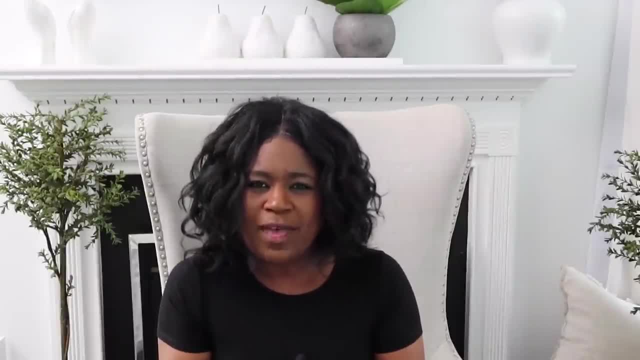 friends, we really need to put ourselves in our kid's shoes. So if you walk by your kid's room and you say, you know, just get your room clean, and it's a disaster. that could be stressful, That could be overwhelming, You know they can start to try to find kind of you know ways to get it. 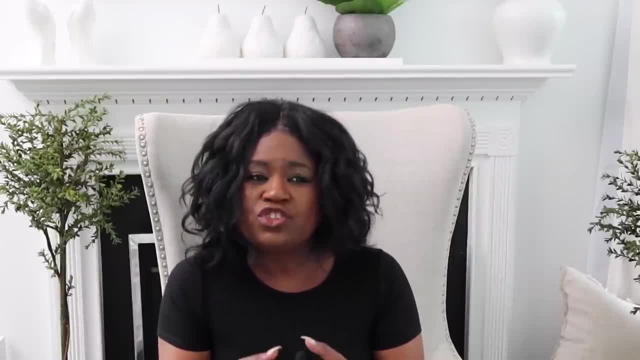 so that you will not fuss, but it's really not clean And it's. it's just like if someone were to tell you, say, your garage is a disaster, and someone tells you: okay, get out there now and clean your garage. When you step out there, you're going to be overwhelmed. It's going to be like 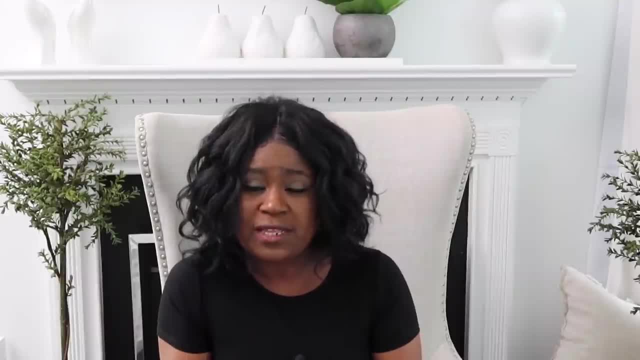 this. This can happen. today. You're going to be stressed And so that's kind of what your kid feels when they are have, they live in a disaster and then they're trying to figure it out. And kids and teenagers they need that guidance and they need for us to approach them. 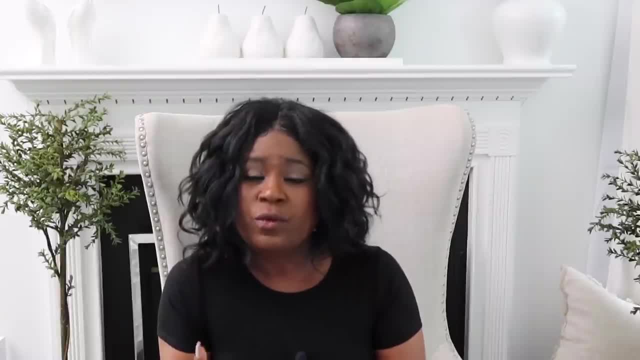 in a way that is motivating, in a way that can really be helpful in a teachable moment for them. So just think about that the next time you kind of run and ask your kid to clean that disaster of the room. If you had to go clean that garage, and what approach would work for you. 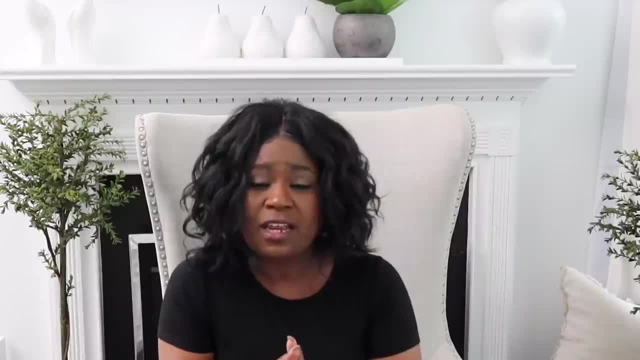 to help you clean the garage. So it may be something like: instead of saying, go out there and clean your garage, I would say: you know what? let's go in the garage and let's find 10 things that we can get rid of today. 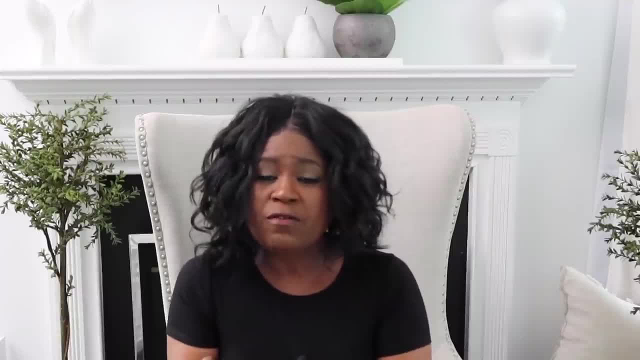 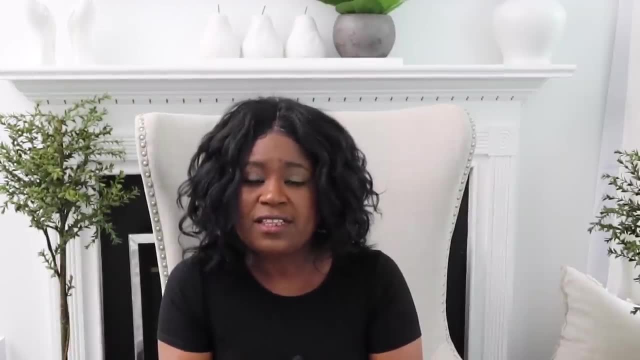 That's a more reasonable request there. So you're biting off the task into smaller tasks. So the same with your kid's room. you know say, Hey, little Johnny, Hey, let's go up your room and let's find 10 things that we can pass on to be a blessing to another child, And so kind of. 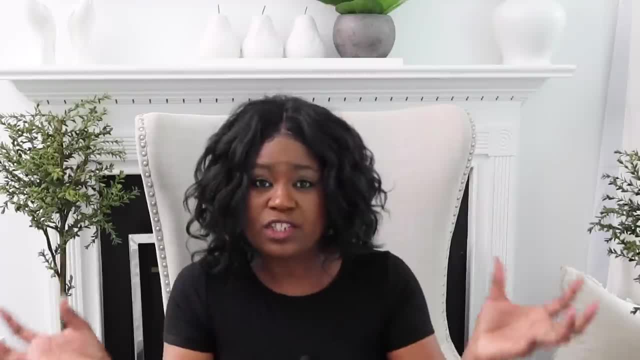 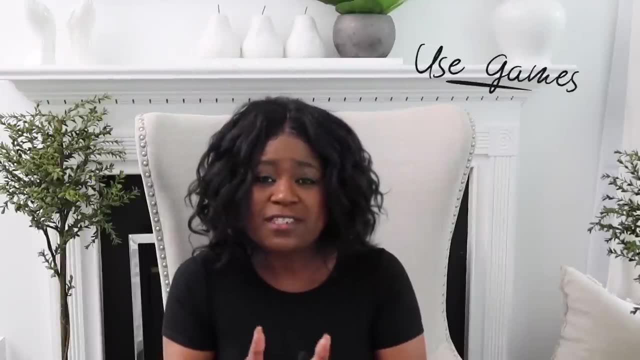 instead of having that big expectation in one kind of swoop, break off the task of maintaining and cleaning their room into little chunks. The next step is to use games. Games can be a such a fun way to get your kid motivated to clean. 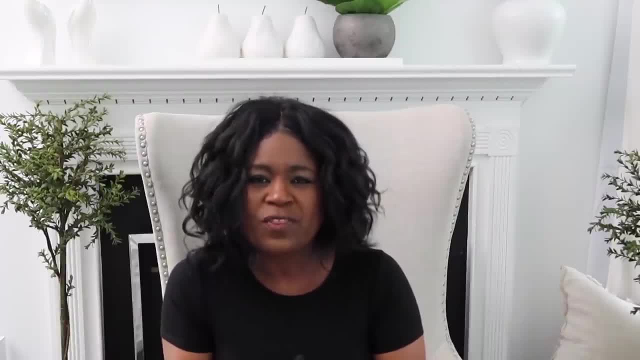 their room. There's so many different cleaning games out there You can do. you can use music with it, but find a way to incorporate the fun with actually cleaning the space, because kids love fun And if you can get um cleaning to be fun for them then it can really help with the. 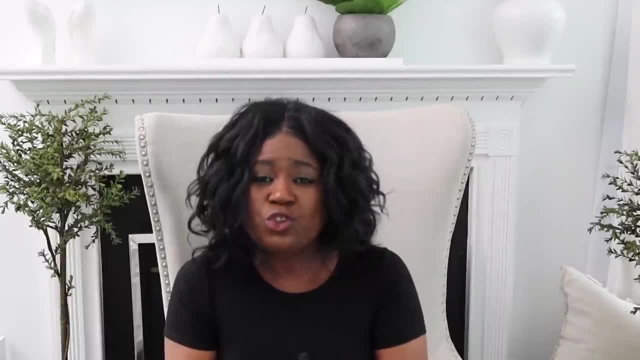 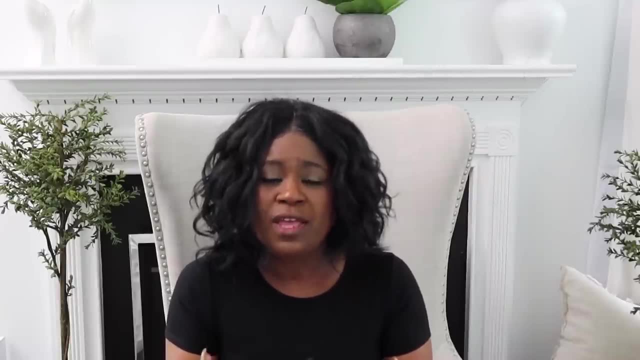 process of them maintaining their space. My next tip is to choose rewards or positive praises when, when they're cleaning their spaces. You know we all love to get positive praises and we love to, you know, hear that we're doing well, And so kids are especially especially responsive to that. 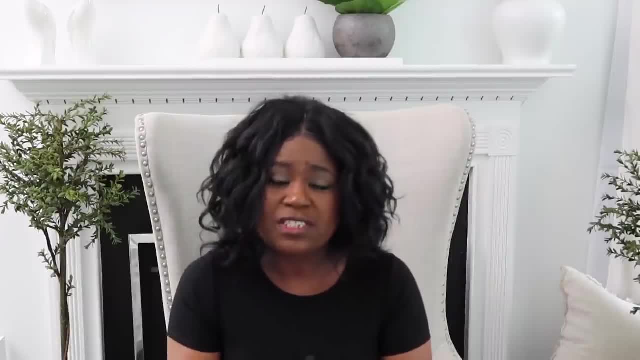 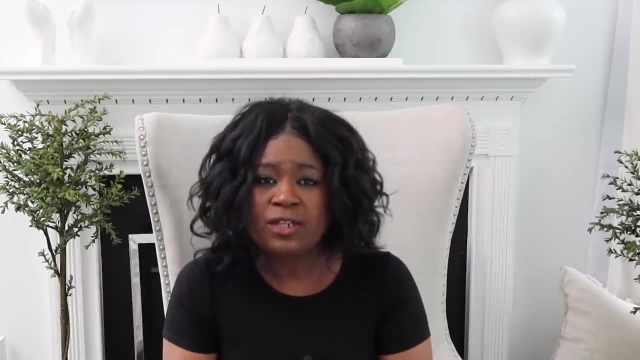 And so one thing you want to do is maybe have some type of reward system in your home, uh, for daily or maintenance, um, of their spaces. whatever you come up with as a family could be a great option. And then also, every time your kid is is doing something well in their space, you know, acknowledge. 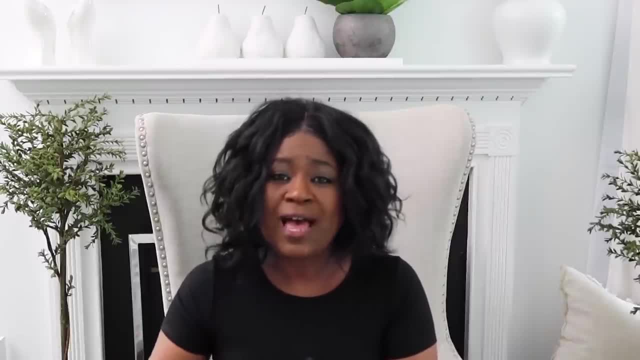 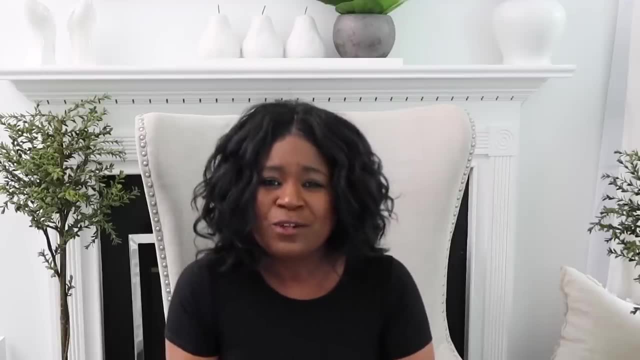 it in a positive way, because that is Going to build the motivation for your child to continue to make you happy by um keeping their space in order. So, friends, the reality is, you know, kids are going to be messy, Some of them. 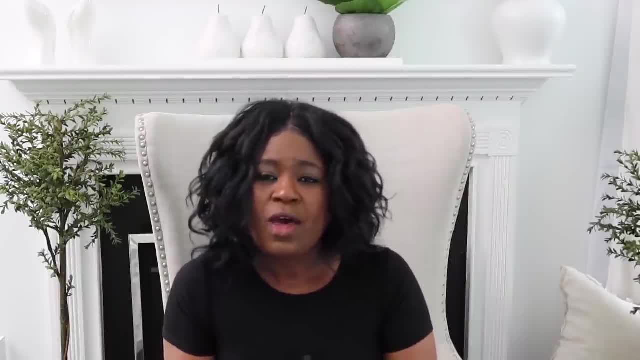 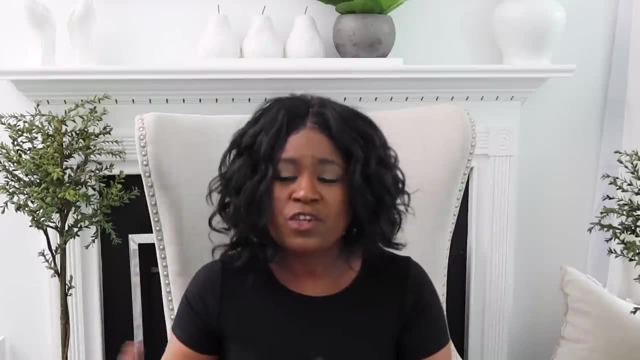 are. they have a lot of things, they have toys, they have books, And so one thing that you kind of want to look at is just to make sure that you're not putting too much stress or too much effort on the mess versus your child, Because we, when we look at this, you have to put the 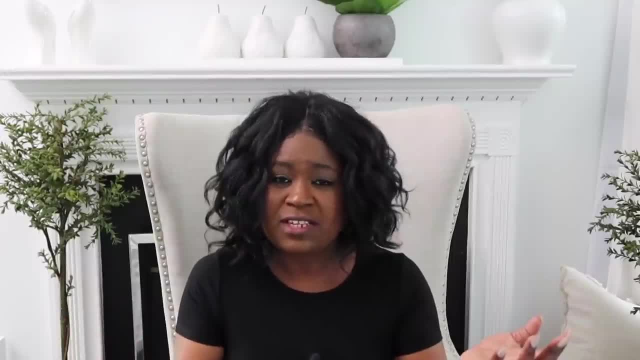 priorities in order. Your child comes in. you have to put the priorities in order. You have to put that umbrella. It comes before the things, And so if you find that you're coming home every day and you're yelling and fussing more than